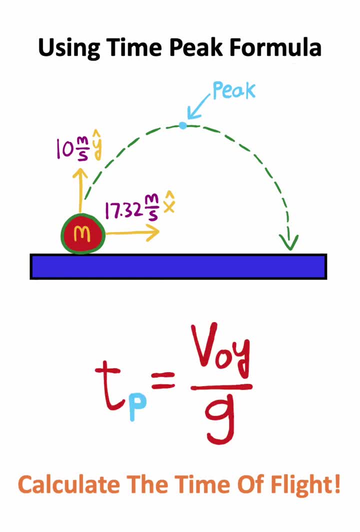 says we are allowed to use the time peak formula, so I'm going to go ahead and give that to you. This formula tells you the amount of time it takes for the projectile to reach its peak. Now to find the time of the whole flight, all you need to do is take this equation. 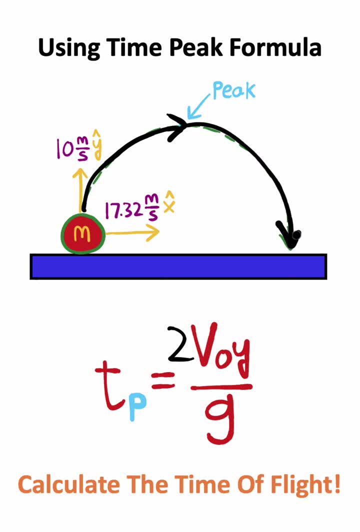 and multiply it by 2, because that will give you the rest of this ball's flight. So now we can plug in the numbers: The velocity in the y-direction is 10 meters per second and gravitational acceleration- assuming we're on Earth- is 9.8 meters per second squared. 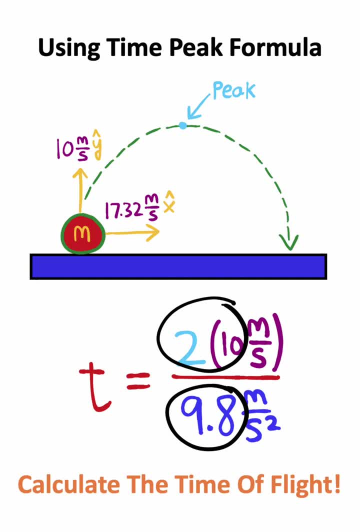 So we have 2 times 10,, which is 20, divided by 9.8.. On a calculator, this is approximately equal to 2.04 seconds, which is the time of flight. Now, this one's a little complicated. but, 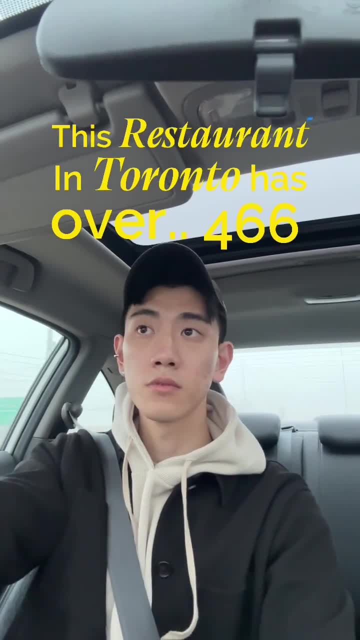 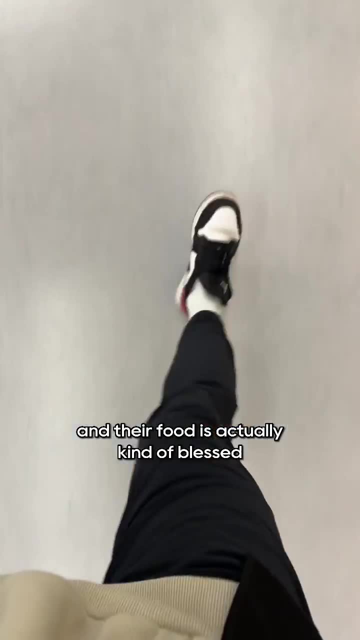 This restaurant in Toronto has over 466 establishments in the world. Okay, you can hardly call this furniture store a restaurant, but today we're going to go eat at Ikea because your boy's broke and hungry and their food is actually kind of blessed. 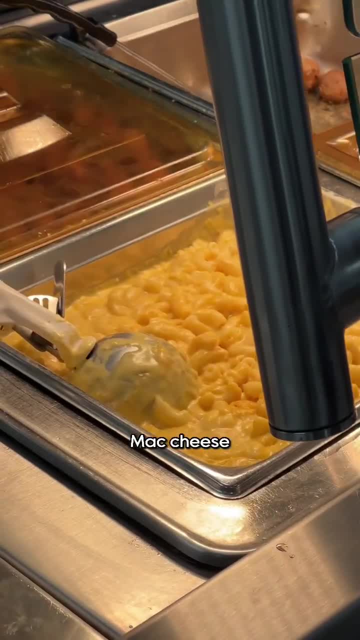 There's actually a wide variety of food options. You have smoked salmon, mac cheese. your fat ass can even get cheesecake too. Okay, hear me out. Ikea butter chicken is actually pretty good, but it wasn't there, so it's pretty sad. 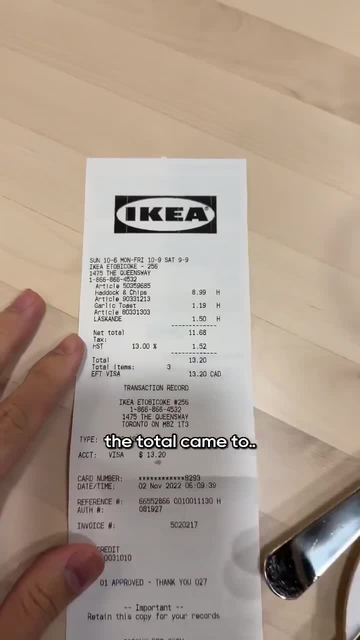 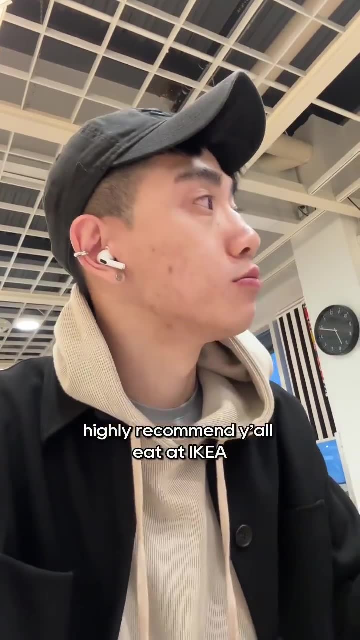 So we settled for fish and chips. I also got a $1 garlic chips, because why not? The total came to $13 Canadian, or for our Supreme Lords and Americans, $9.75.. The food is pretty good, nothing special. I recommend y'all eat at Ikea. 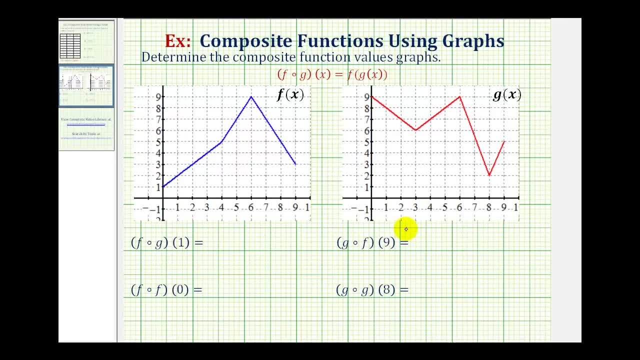 We want to determine the composite function values from the graphs of function f in blue and function g in red. From this definition here we see there are two ways to express a composite function. I think it's going to be helpful to rewrite these composite functions using the notation given here on the right. 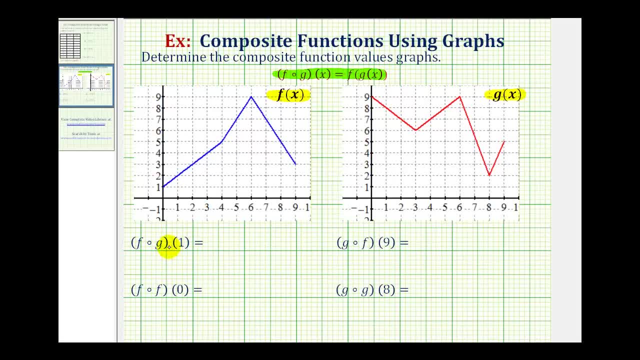 So for f of g of one or f after g of one, we can write this using this notation here. For g of f of nine or g after f of nine, we can write using this notation here. For f of f of zero, we can write like this: